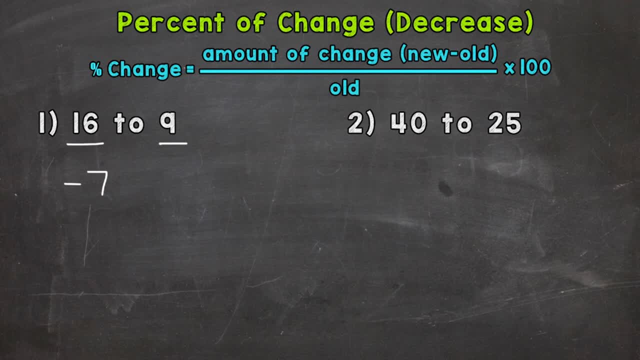 a negative number because we started with 16 and now we have a 9. So that negative represents a decrease. Let's divide by the old number, which is 16. And we need to multiply by 100. So we have a negative 7 divided by 16.. That's going to give us negative 4,375, ten thousandths, And we multiply. 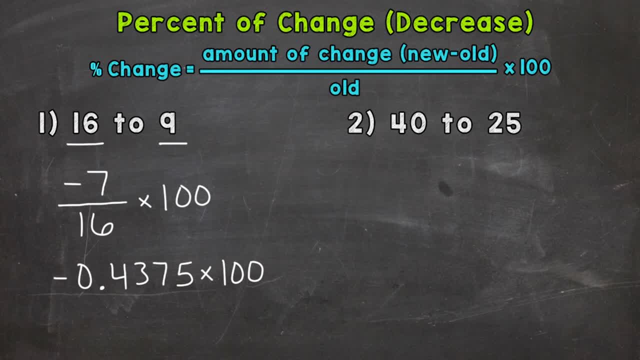 that by 100.. Before I do that, I do want to mention that you have to make sure to always divide by the old or original number, Because that's the number that changed. So we want the percent, The percentage change relative to the number we started with. We're looking at the percent that that. 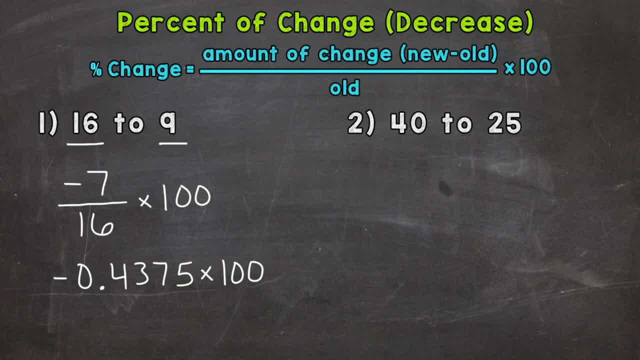 number changed. Alright, let's multiply by 100.. Now, when we multiply a decimal by 100, we can just move the decimal twice to the right, So 1,, 2. And we end up with an answer of negative 43.75 percent. And 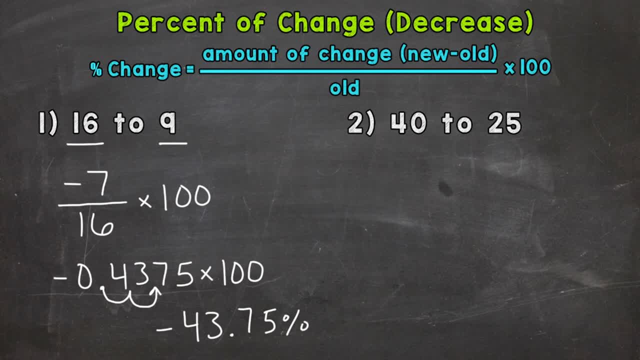 again that negative represents a decrease. So we can express this answer in two ways. We can say negative 43.75 percent And again that negative represents a decrease, Or we can write 43.75 percent decrease. So here is one way to express our answer And here is the other. 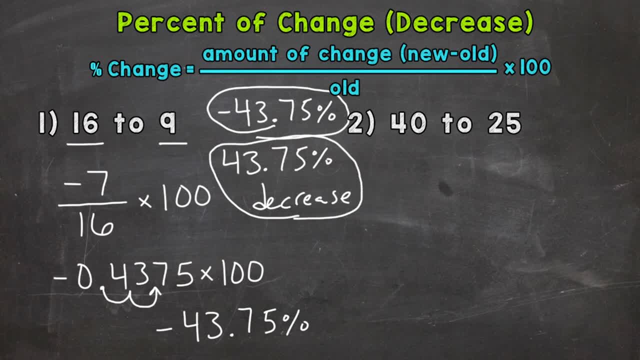 So using a negative to represent the decrease, or writing decrease out. Let's move on to number two, where we have 40 to 25.. So the first thing we need to do calculate the amount of change. So the new number 25 minus the. 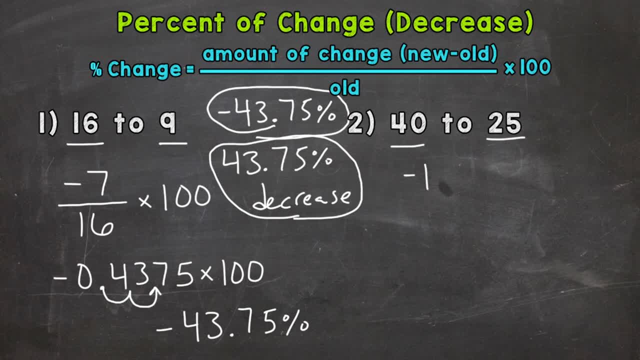 old 40. So we get negative 15.. Divide by the old number of 40. And then we multiply by 100 to convert it to a percent. Remember always divide by the old number. So negative 15 divided by 40 is going to give us negative 375 thousandths.